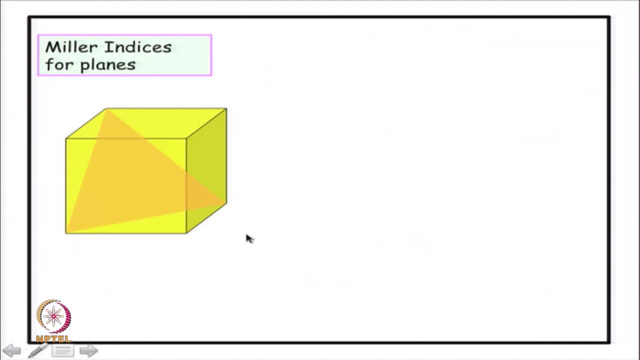 here which is passing through three corners of the unit cell and we want to specify, give a name or give a Miller indices to this plane. So, like in the direction, we have to choose an origin and a coordinate system, the crystal coordinate system, and recall that the crystal, 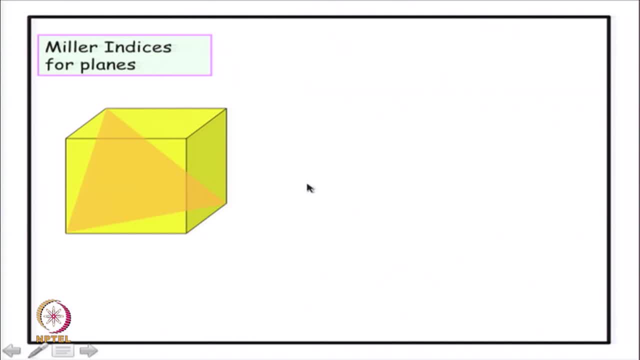 coordinate system has its edges parallel to the unit cell edges, But one difference is there. when we talked about the direction, we said that the origin should be so chosen that it lies on the direction. The origin for the direction is lying on the direction. 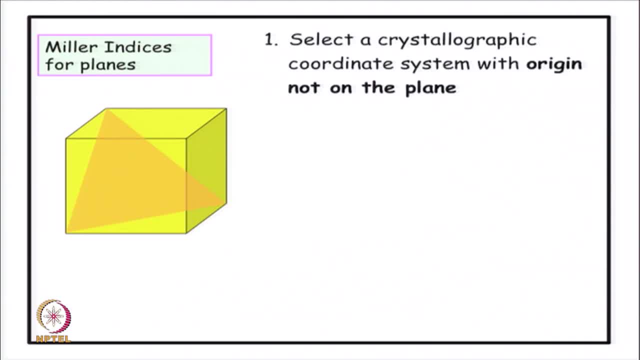 but in the case of plane, just the opposite is true. So we have to select a crystallographic unit system with origin not on the plane. This point has to be kept in mind. It will become obvious why this requirement is there. So we choose a origin here, in the back corner. 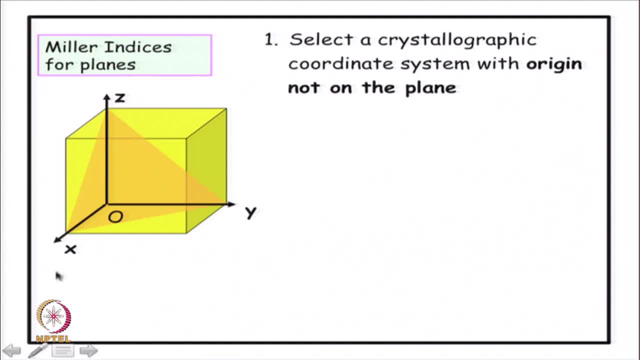 which is not one of the corners through which this plane is passing, and we set up the x, y and z axes, which are parallel to the unit cell edges. So this is the first step, And it is an important step. Beginners can make a mistake by choosing origin on the plane. 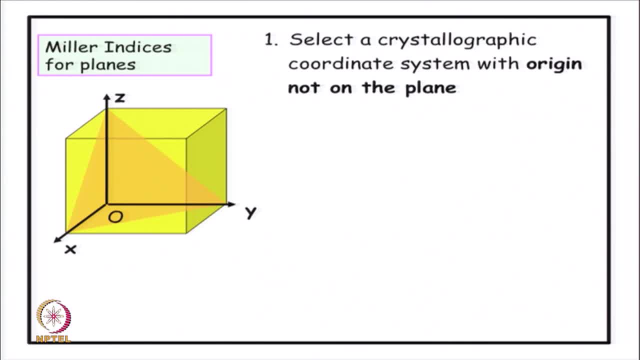 We have to keep in mind that origin should not lie on the plane. if we are trying to find the Miller indices of the plane, The second step is find the intercepts along axes in terms of the respective lattice parameter. So this plane is intersecting the x axis. 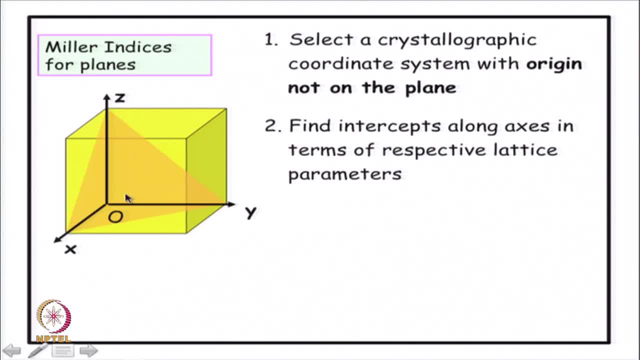 at the unit cell corner, So which means it is intersecting at a distance, a. a is the edge length of the unit cell along the x axis, But we will show this as 1, because we are trying to write the intercepts in terms of respective lattice parameter. So, in particular, 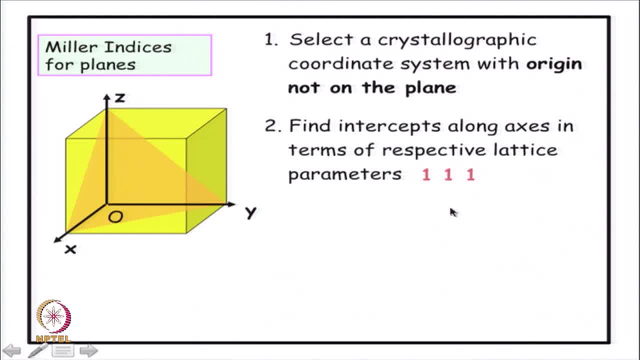 for this plane. I have so selected that all the 3 intercepts are 1, 1.. So we have to write 1, 1, 1 as the 3 intercepts. The first intercept one says that the plane is intersecting. 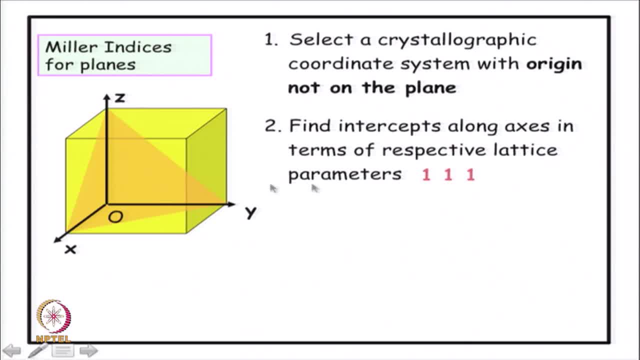 at a distance a from the origin. The second one tells us that it it is intersecting at a distance b from the origin, and the third at the distance c from the origin. Then we have two more steps for completeness. We write it here, although we do not need it immediately. 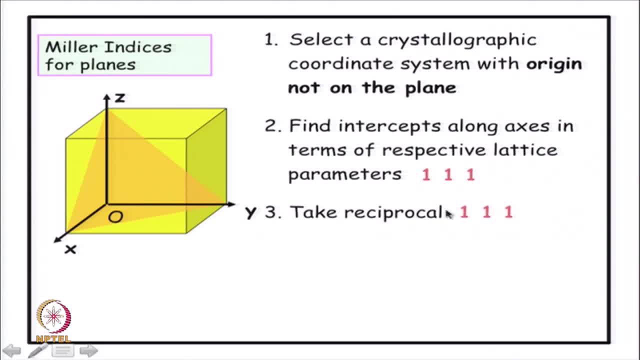 And it is an important step For completeness. we write it here although we do not need it. intercept that the intercepts are then reversed or you have to take the reciprocals of the intercept. So intercepts directly are not taken as Miller indices, but the reciprocal. 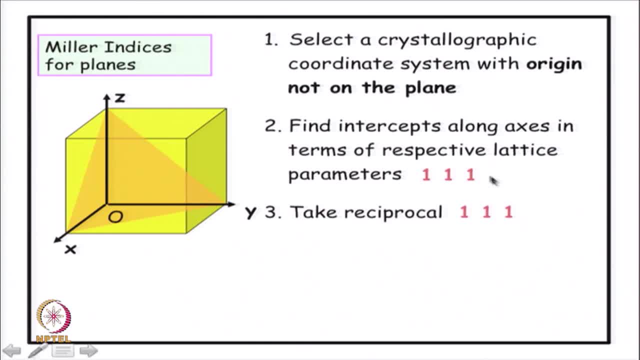 of the intercepts are taken as Miller indices. In this case, of course, it is trivial because we have started with a simple plane all of whose intercepts are 1, 1, 1.. So taking the reciprocal it is still gives me 1, 1, 1.. The fourth step is to convert again them into 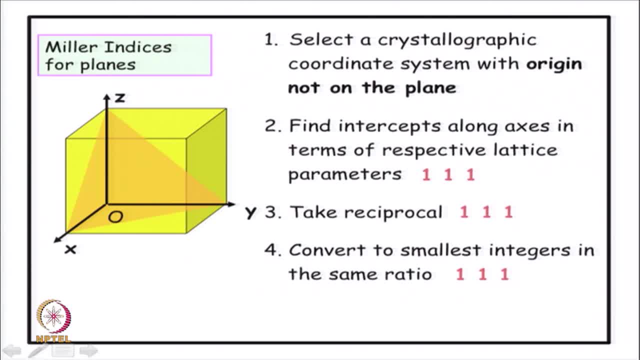 small integers having the same ratio. We had this step for the direction also, the same step we repeat here for planes as well. So if we had any fractions or if we had any common factor, we would have cancelled them suitably by multiplying or dividing by some number. 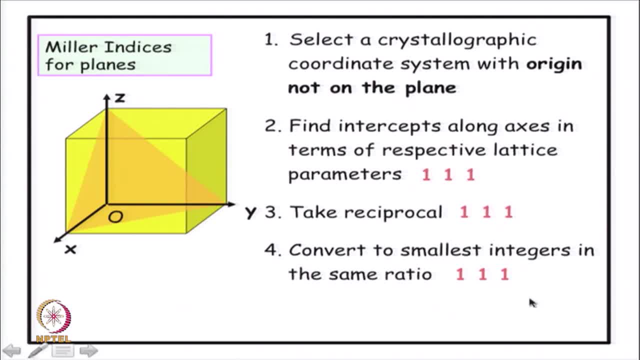 So, again, that is step is not relevant here for this example, So we simply write it as 1 1, 1.. The final step, again an important step, is to use the correct bracket, and in this case we use parenthesis, that is, the round brackets For direction. remember we used square bracket. 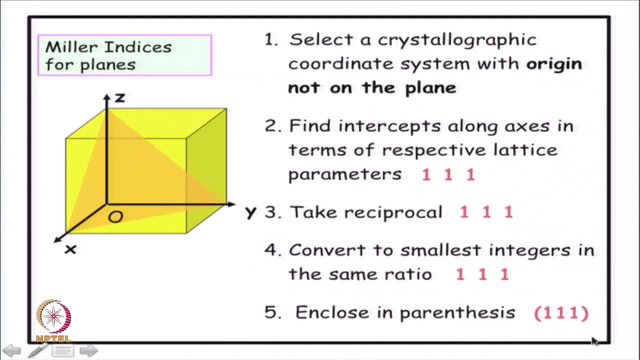 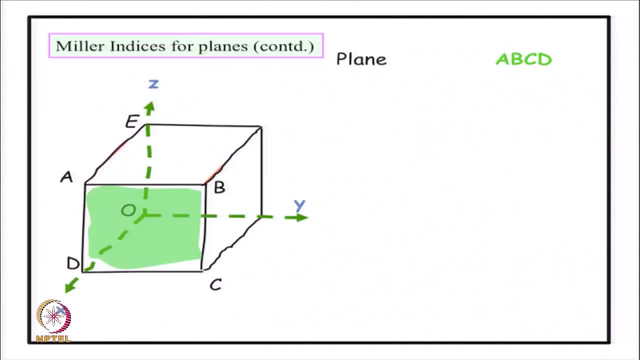 now for planes we are using round bracket. these conventions we need to follow. Let us now look at another example. So now we want to index this front face of the unit cell, the plane, a, b, c, d. So we choose an origin. on the back face corner the x, y and. 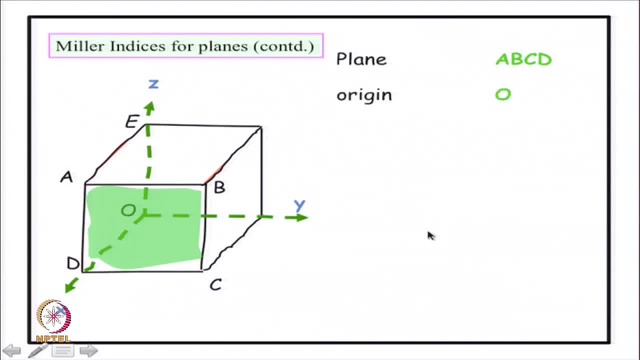 z axes are there. So origin at o, not lying on the plane. and then we find the intercept. Look at this plane. it is intersecting the x-axis over of the, for that mean axis at 1 or a, So the x intercept is 1, but this plane being the front face of the 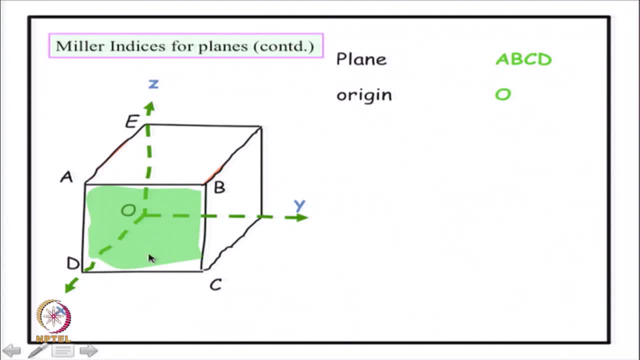 unit cell is parallel to the other two axes, So it is parallel to y and parallel to z. and whenever a plane is parallel to any given axes, we by convention take the intercept as infinity. So if the plane is parallel to axis y, we assume that it is intersecting. 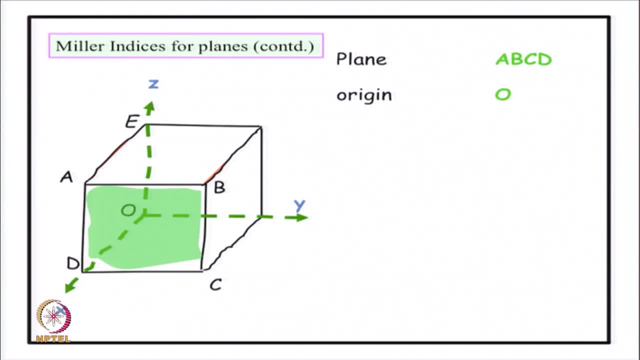 the y axis at infinity. So we will write the intercepts here as 1 for the x axis and infinity for both y and z, because it is parallel to both y and z. Now taking the reciprocals become relevant, because when we take the reciprocals we are 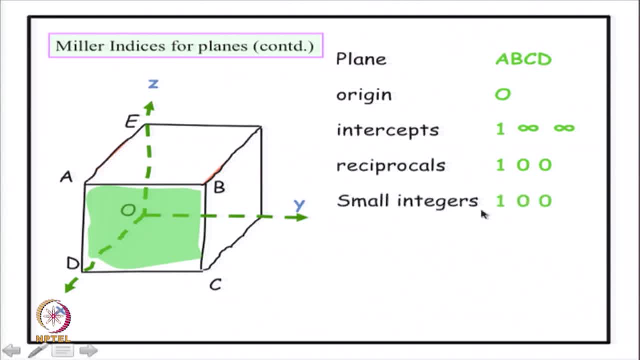 taking the reciprocals of infinity. we put zeros and finally they taking it into a small integer. it is already a small integers. there is no common factor or there is no fraction, So I still get 1, 0, 0 and finally the Miller indices. I put the round brackets to define. 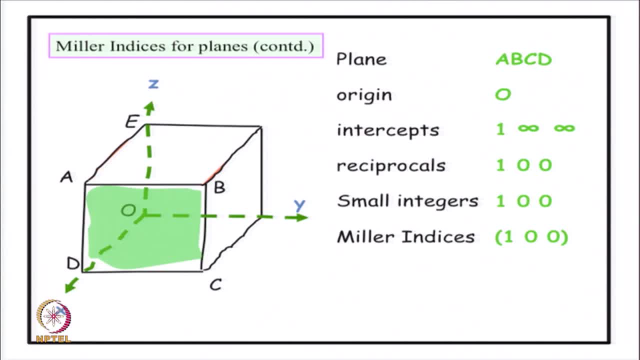 that it is Miller index of a plane. So this green plane will have the Miller indices 1 o o. Thank you. 1 0, 0. And please note that 0 corresponds to 0 in the Miller indices correspond to infinity. 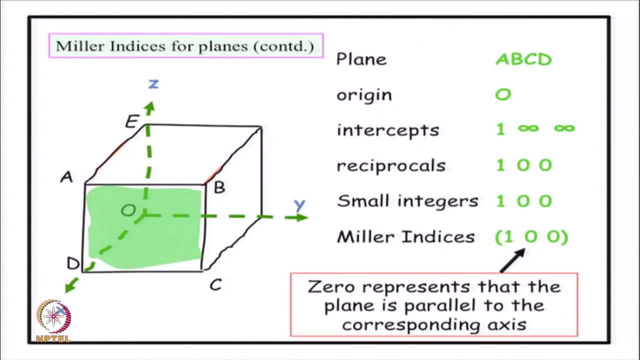 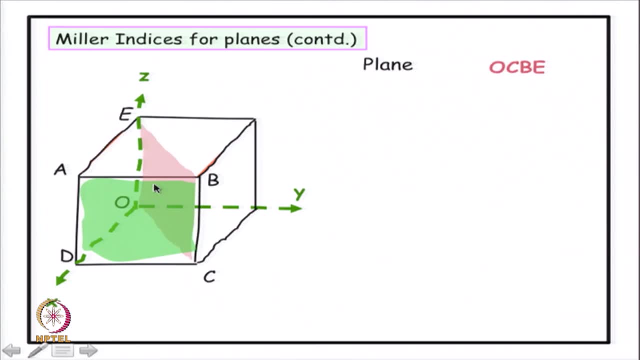 in terms of the intercept, and infinity in terms of intercept means the plane is parallel to that axis. So a second 0 means that the plane is parallel to the y axis. the third 0 means plane is parallel to the z axis. Now let me introduce another plane, which 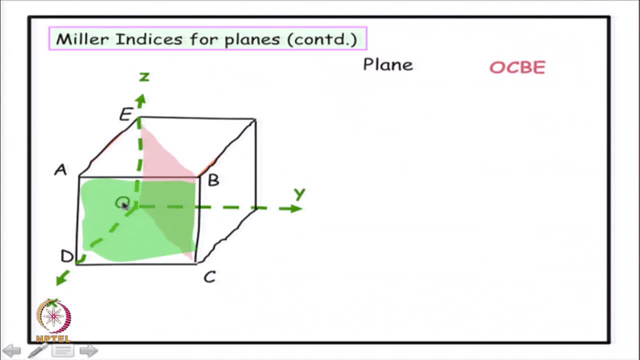 is a more infinite energy relation, corresponding to infinity х. So let me introduce another plane in the same unit cell, yay, This time the plane obce. Now, this plane happens to be passing through my chosen origin. So the first condition, the very first condition: that plane should not pass through the origin. 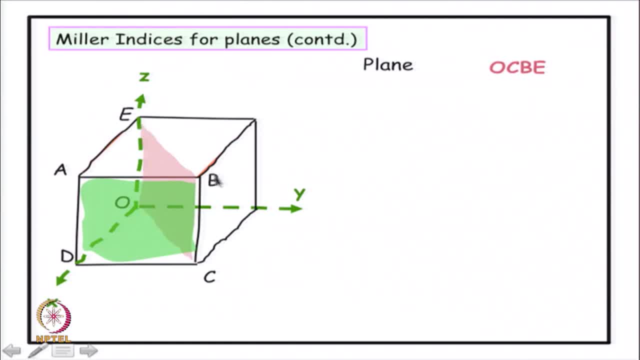 is being violated Right, which is not passing through the plane or which is not lying on the plane, So I shift my origin to this corner. Please note that when I am shifting the origin to this corner, I am keeping the axes parallel. This is what we had done for the directions also, and the same procedure has 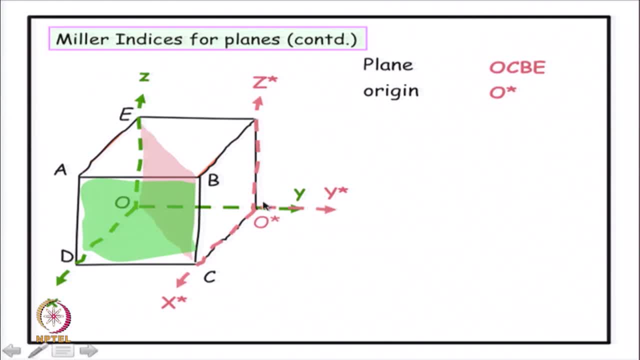 to be repeated for planes as well. So we are free to choose the origin anyway, But once for a given problem. if we have chosen the axis orientations, then the same axis orientation has to be followed with the new origin. So my x star axis is parallel to x, the y star. 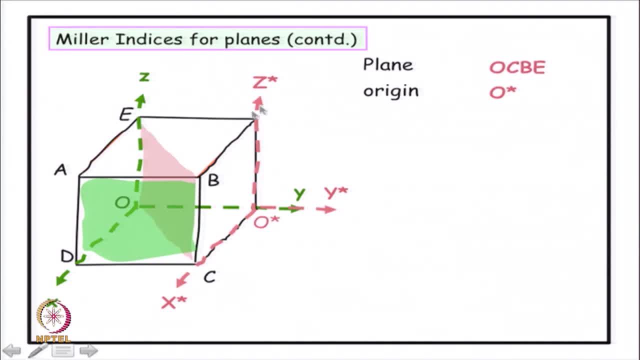 axis is parallel to y and the z star axis is parallel to the z direction, Because I want to relate the Miller indices of this new plane to my original plane. a, b, c, d, So the intercepts now, on the x axis, the intercept is: 1.. On the y axis, if I move in the positive 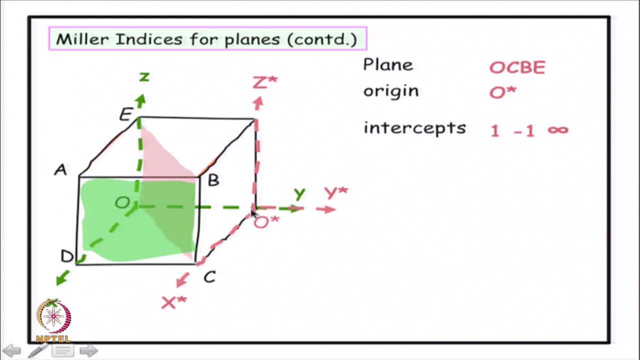 direction. there is no intercept. To get the intercept on the y axis I have to move in the negative direction. So I have a negative intercept in the y axis and it is the plane is still parallel to the z axis. So the third intercept is infinity. We now take the reciprocals So we get 1, minus 1. 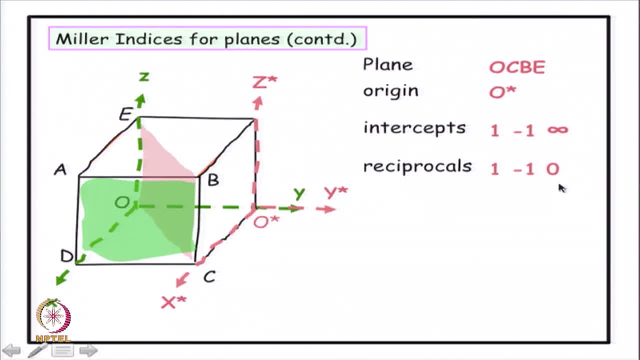 and infinity. the reciprocal is taken as 0.. We now put the Miller indices into round brackets and, just like for the direction, we write the minus as a bar over the number. So wherever we have bar means 0. This means we have a negative intercept. 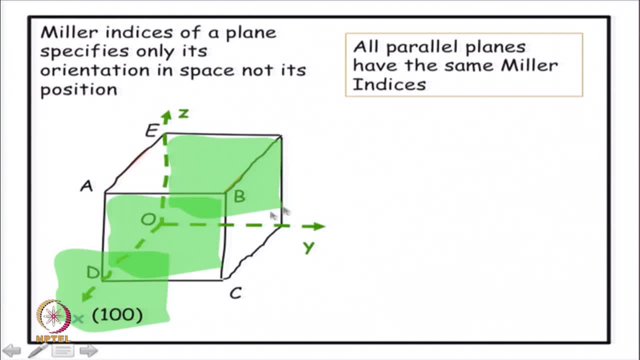 Let us make this point that whenever we write Miller indices of a given plane, actually it is not representing only that plane but all parallel planes. So Miller indices of a plane specifies only its orientation in space and not its position. It can be any plane parallel. 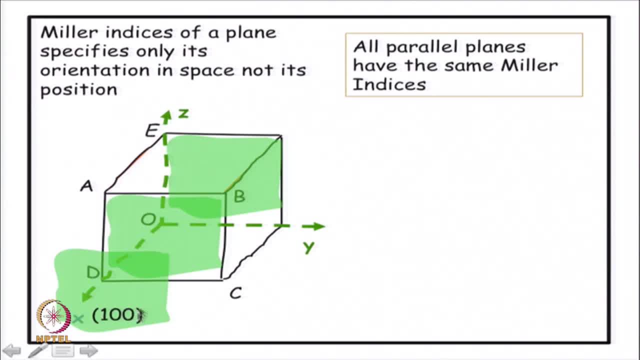 to a given plane. So when I say 1 0, 0, I did it for the front face of the unit cell, but the back face also will become 1 0, 0 and all faces parallel to this will be 1 0, 0. So all parallel planes. 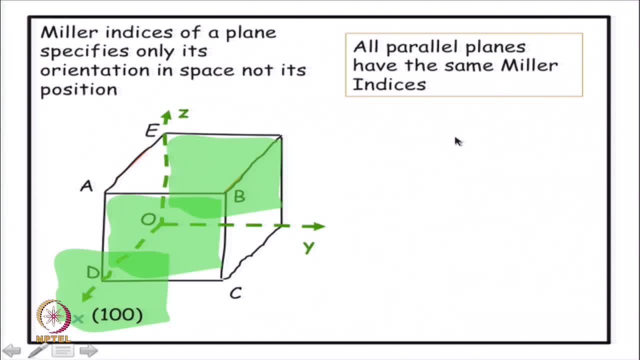 have the same Miller indices And in fact we also have the convention that if all indices are multiplied by minus 1, that if all of, Instead of the indices are multiplied by minus 1, that if all of, instead of the indices are multiplied by minus 1, that if all of, instead of the indices are multiplied by minus 1, that 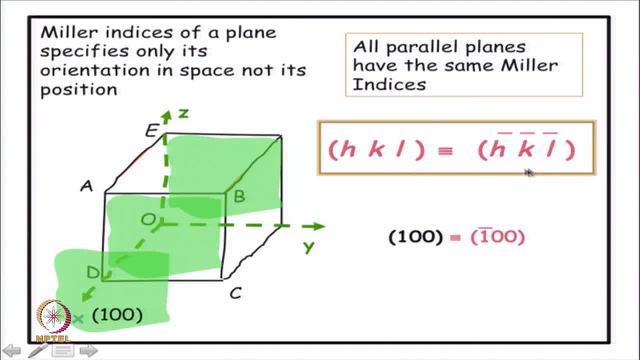 these h, k, l. if we take the negatives of them- minus h, minus k and minus l, or bar h, bar k and bar l- then they represent the same plane. This is true because we are free to choose the origin and these two indices depend on which side of the plane we have chosen the origin. Note that any plane will divide the 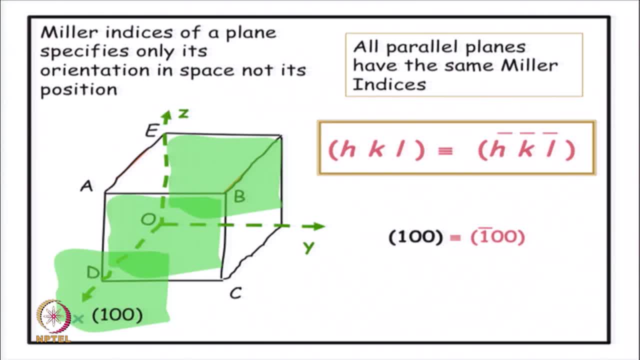 space into two halves. We are not allowed to choose the origin on the plane. we can only choose the origin on one side, one half of the plane or the other half of the plane. So when we choose the origin on one half space, we will get one set of indices and if we choose 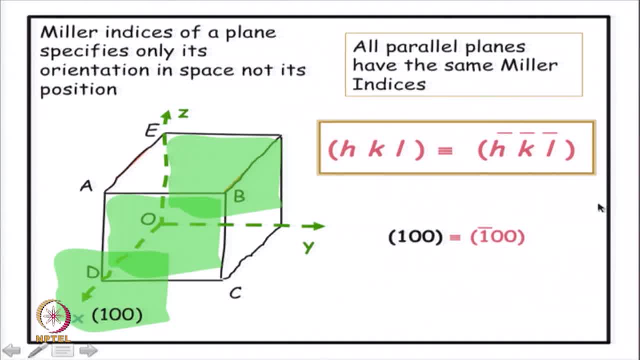 the origin. on the other side, we will get the negative indices. So, for example, the 1 0, 1 0 0 and bar 1 0 0 actually represent the same plane. There are situations in which we may like to distinguish between these, but this is the. 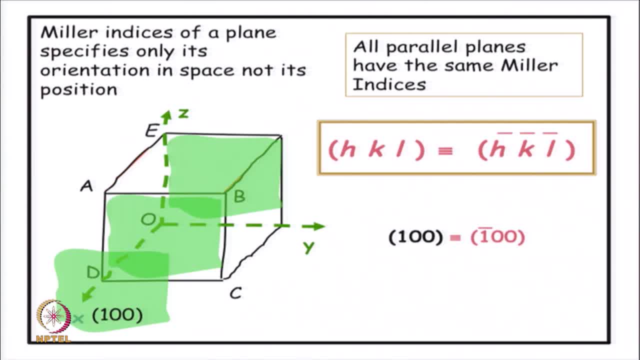 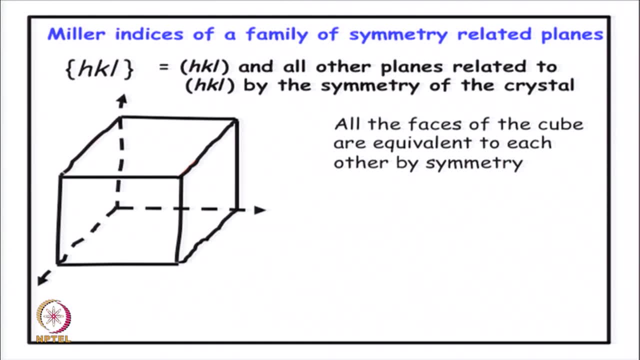 useful convention. Now, just like we saw that there are symmetry related directions and there was of interest to represent them by one set of Miller indices. All symmetry related directions, Similar convention or several similar requirement is there for Miller indices of symmetry related planes. So if we have a set of symmetry related planes then we put them. one of the indices we put. 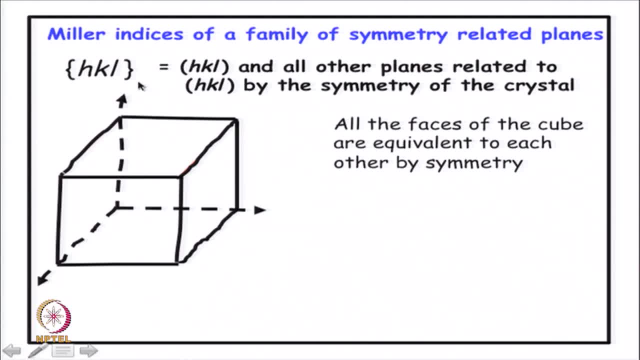 them in angular brackets. sorry, not angular bracket, curly bracket. So if we, if you use this curly bracket, it represents not only the hkl plane but all other planes. So we can see that the hkl plane represents the same plane as the other planes related. 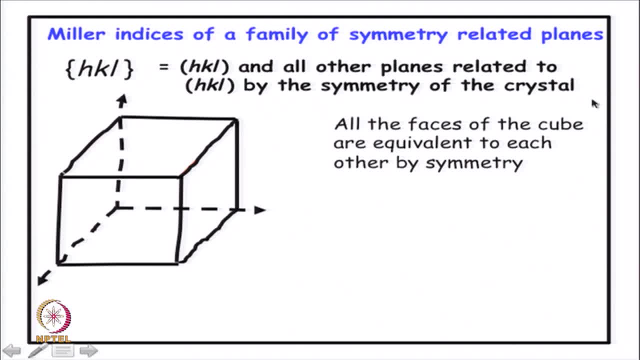 to hkl by the symmetry of the crystal. So for example, we know that by symmetry, if I have a cubic unit cell, by symmetry all faces of the cube are equivalent. They are symmetry equivalent because they are symmetry operations of the cube which will take one face to the other. 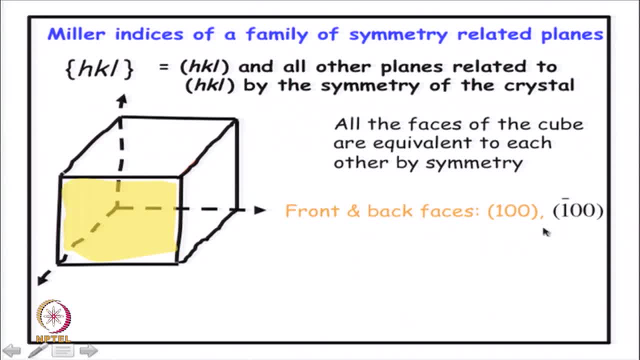 So let us look at the front and back faces. So we have 1 O O and bar 1 O O. Then we have left and right faces, So this is O 1 O and O bar 1 O and finally the top and bottom faces: O O 1 and O O bar. 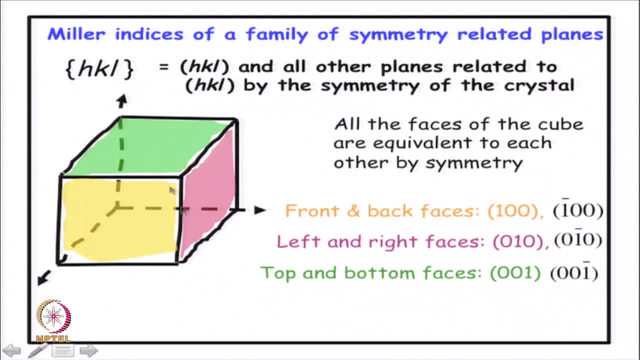 1. And if we want to represent all these planes in one set of Miller indices, I pick up any of these 6 as the representative member And put it in the central axis in the angular bracket. So if I put 1 o o, if I pick up 1 o o as the representative of 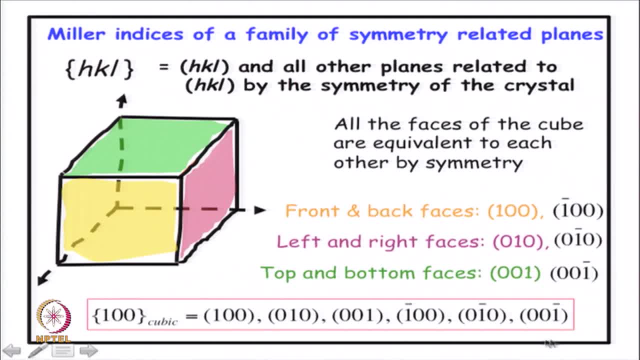 all these planes, then it means any of the 6 indices: 1 o o, 1 o o, 1 bar, 1 o o o bar, 1 o and o o bar 1.. Recall that since these are representing symmetry related planes, the meaning of this index- symmetry related direction index, the family index- will depend upon what crystal 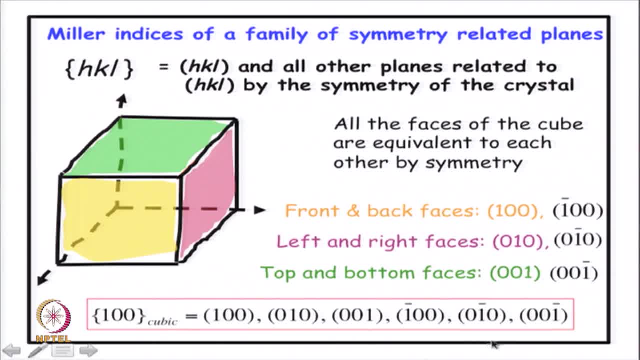 symmetry we are talking about. So this equivalence which we have written here is only for cubic, and that is why I have given the subscript cubic to 1 o o. For other crystal systems it is not necessary that 1 o o will mean all these 6 indices. 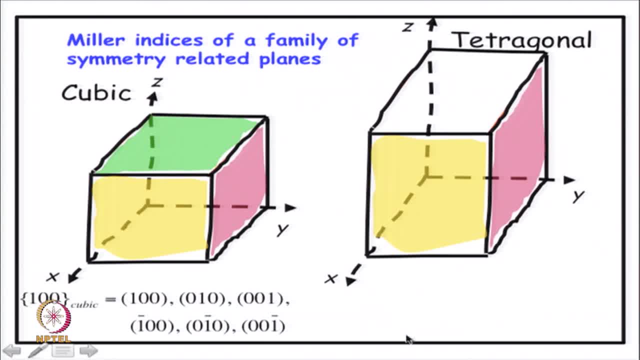 we will take up an example. let us consider the tetragonal. We have already seen that 1 O O cubic means these 6 indices. but what about 1 O O tetragonal? 1 O O tetragonal in. 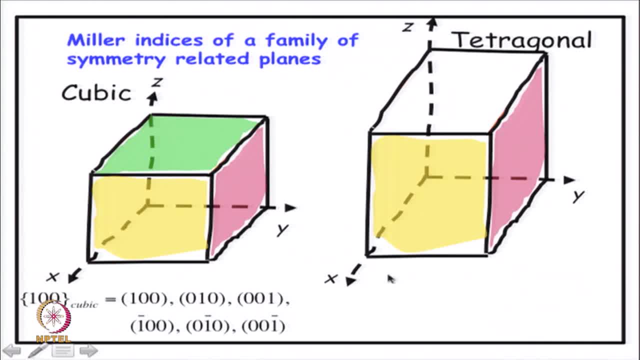 terms of the face is the front face of the tetragonal unit cell. this face, the yellow face. but tetragonal has a 4 fold symmetry axis parallel to the z axis. So all the vertical rectangular faces are equivalent. so 1 O O the yellow face is equivalent. 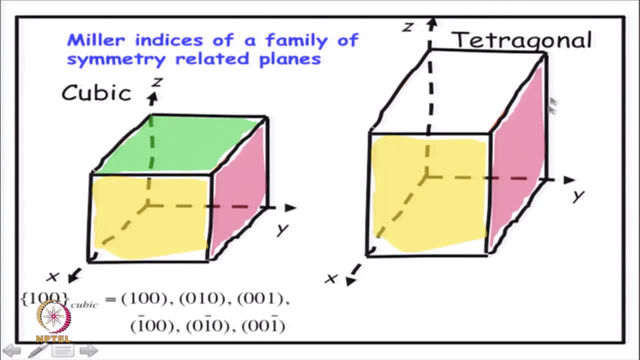 to 0, 1 O, which is the red face here, But then the horizontal face, the base or the janganism vedere. istagne is basically a vertical Free shape of a钩固形形 of a seeming of the tetragonal unit cell, or the roof of the tetragonal unit cell is the 001 plane. 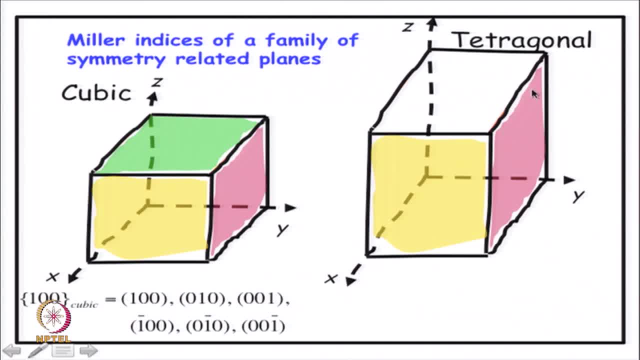 This is a square phase and this is not equivalent. there is no symmetry operation of the tetragonal system which will take this vertical phase into a horizontal phase and geometrically we can see that there cannot be any mapping of a rectangle to a square. So there is no symmetry. by symmetry, the horizontal phases are different from the vertical phases. 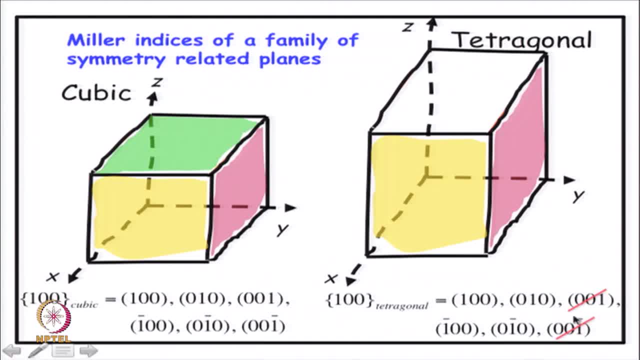 so when I say 100 tetragonal, the horizontal phases are not member of that family. So we will have only four indices now: 100, 010, bar 10 and 0 bar 10.. I have cancelled 001 and 0 bar 1, which represent the horizontal phases which were member of. 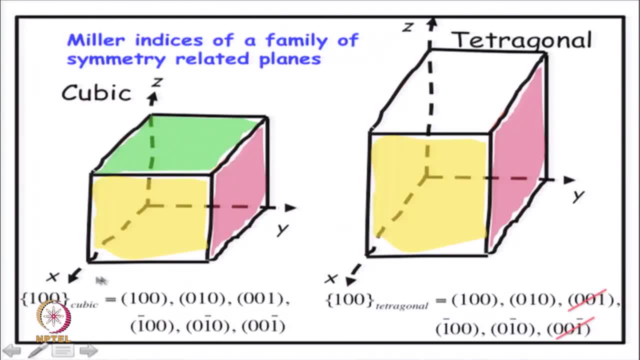 that number when we were talking about- sorry, when we were talking about- the cubic family, but in this situation they are in the tetragonal system. they are not equivalent. So it is important to keep this in mind. sometimes one makes a mistake to assume that always 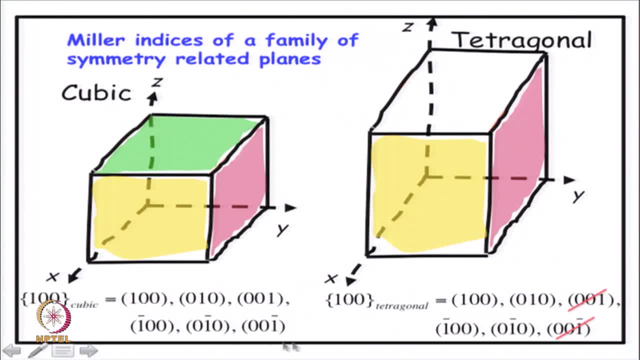 any permutation of the number given will represent the family. This will be true only for cubic system, because in cubic all three edges are equivalent, So the numbers corresponding to those edges can be permuted. In other systems we have to be careful. so in tetragonal the x and y were equivalent.